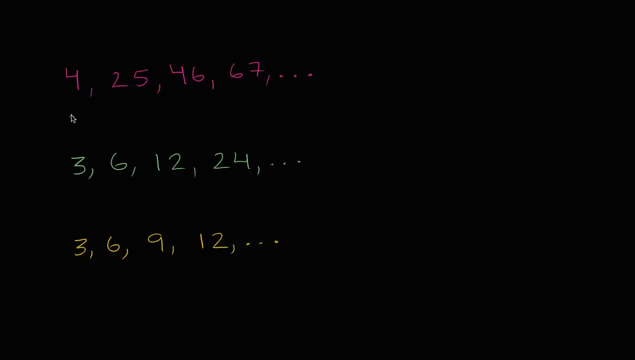 What I want to do in this video is get some practice figuring out patterns in numbers and in particular, patterns that take us from one number to a next number in a sequence. So if over here, in this magenta color, I go from four to 25, to 46, to 67,. 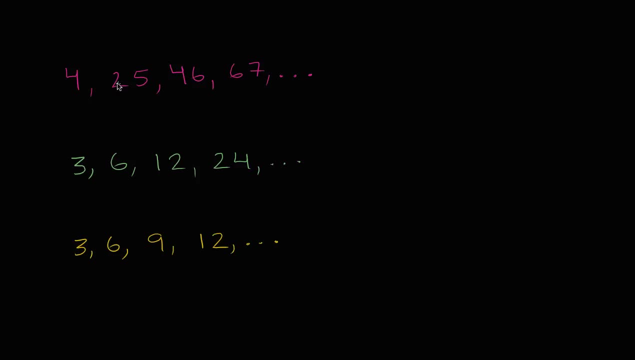 so what's the pattern here? How did I get from four to 25, and can I get the same way from 25 to 46, and 46 to 67, and could I just keep going on and on and on? Well, there's a couple of ways to think about it. 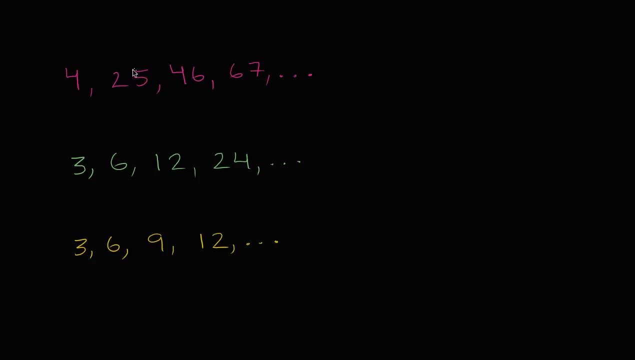 When I see four and 25,, let's see 25 isn't an obvious multiple of four. Let's see another way to go from four to 25, I could add 21.. So let's see if I add 21,. 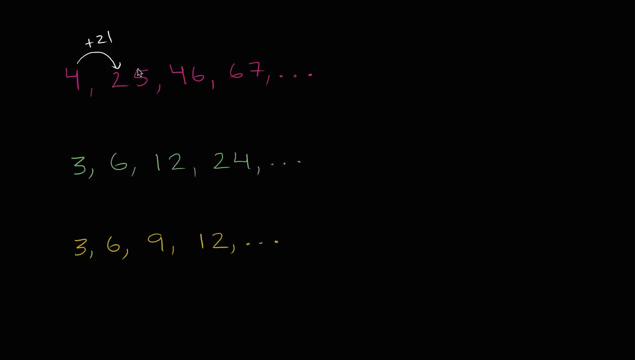 four plus 21 is 25.. Let's see if I were to go from 25 to 46, well, I could just add 21 again. So it looks like to go from one number to the next. I'm just adding. 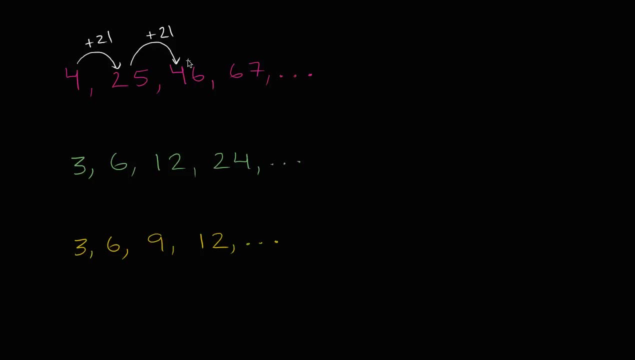 I'm just, I wrote 12 by accident, 21.. I'm just adding 21 over and over again, So that's going to be 46 plus 21 is 67. And if I were to keep going, if I were to keep going, 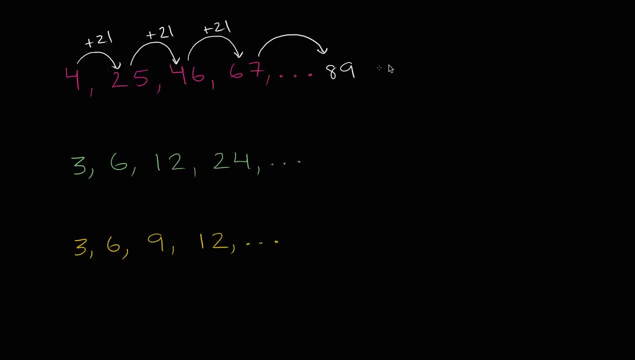 let's see: if I had 21,, I'm gonna get to 89.. If I add 21 to that, I'm gonna get 100, and I'm just gonna get 110, and I could keep going and going, and going. 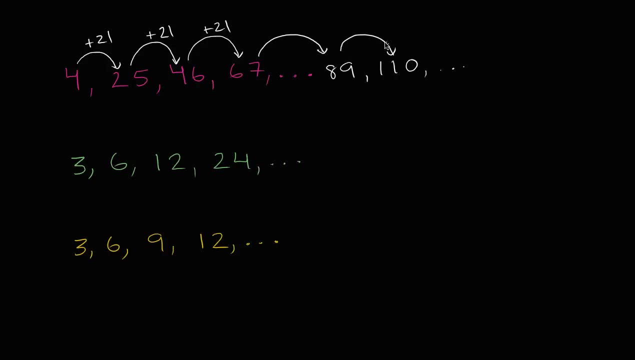 I could just keep adding 21 over and over again. So the pattern here is: I am adding 21.. Now, what about over here in green? Well, when I look at it at first it's tempting to say, okay, three plus three is six. 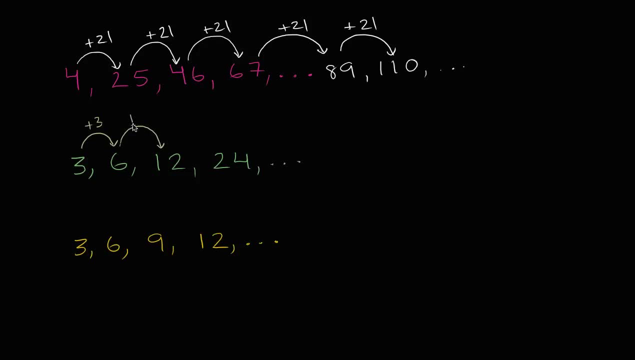 but then I'm not adding three anymore. to get from six to 12, I'm adding six. And then to get from 12 to 24, I'm not adding six anymore, I added 12.. So every time I'm adding twice as much. 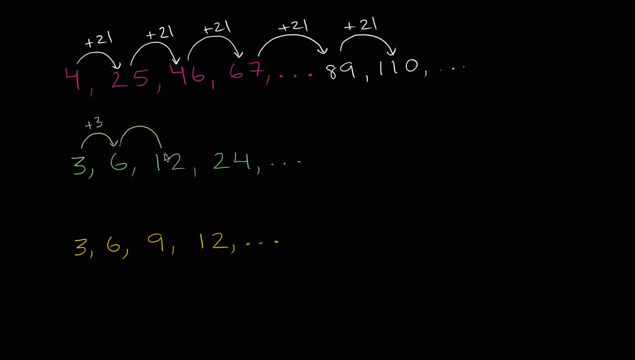 But maybe an easier pattern might be. another way to go from three to six isn't to add three, but to multiply by two. So I multiply by two to go from three to six, and if I multiply by two again, I go from six to 12.. 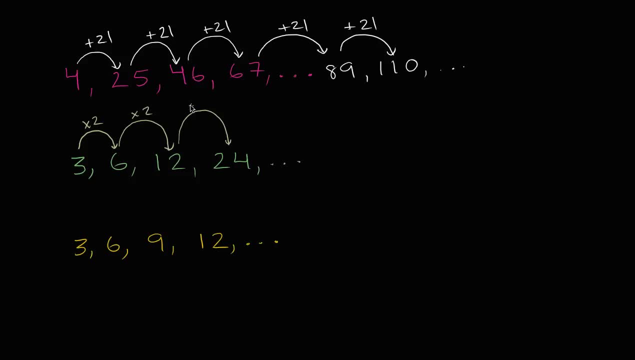 Six times two is 12., And if I multiply by two again, I'll go to 24.. Two times 12 is 24, and I could keep going on and on and on. Two times 24 is 48, 96..